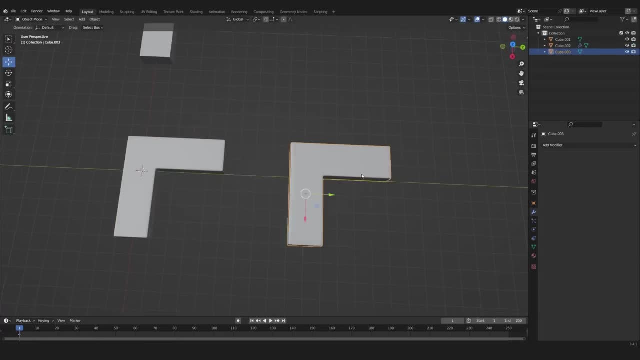 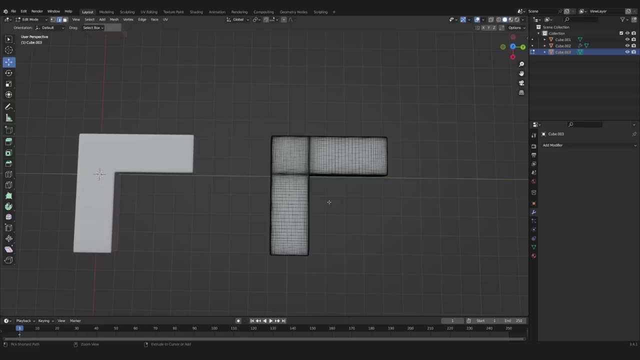 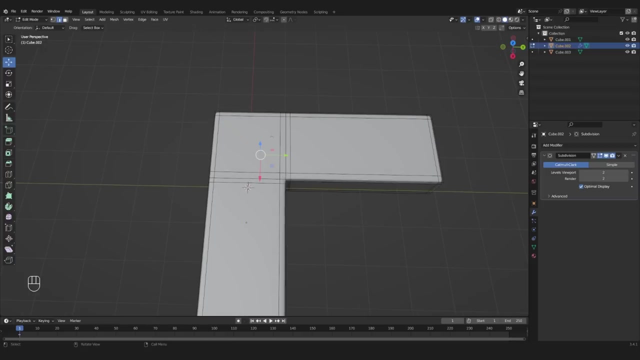 Also, if we apply the modifier, you can see that the tessellation is much more dense in these areas, which might cause problems when adding a displace modifier or deforming the mesh. Luckily, there's an easy fix to that In edit mode. press K for the knife tool and cut a diagonal edge from the corner. 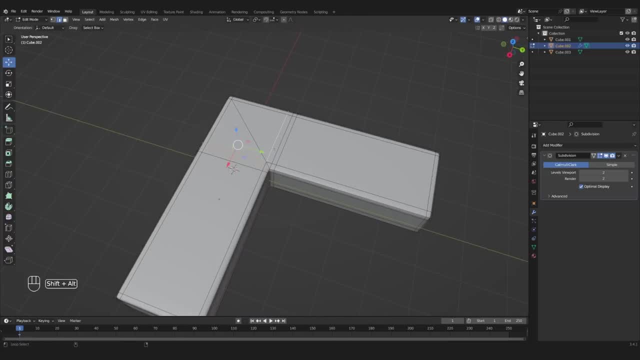 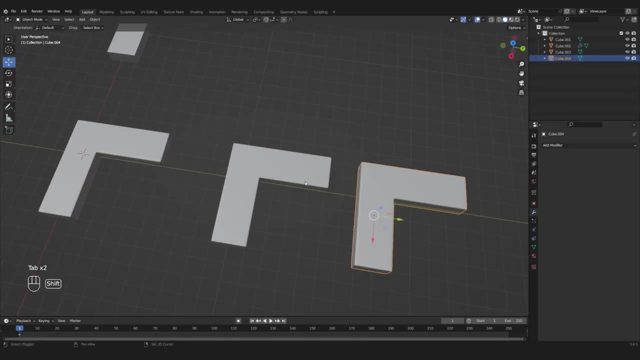 like this: You can now delete the inner edge loops on both sides. Now your edge work goes around the corner. When applying the subsurf modifier, the tessellation is much more even. Here's an example on where I used this method, As you can see, 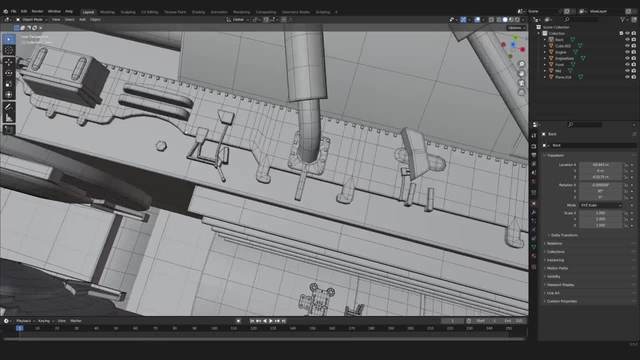 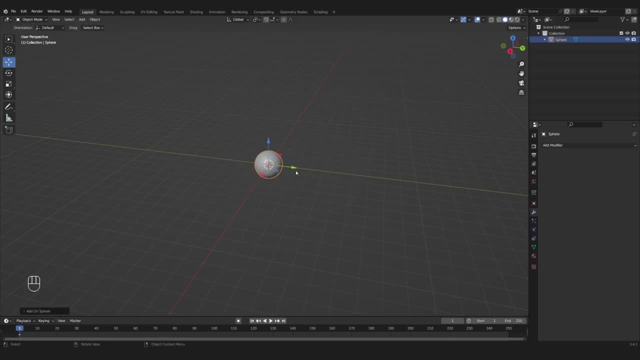 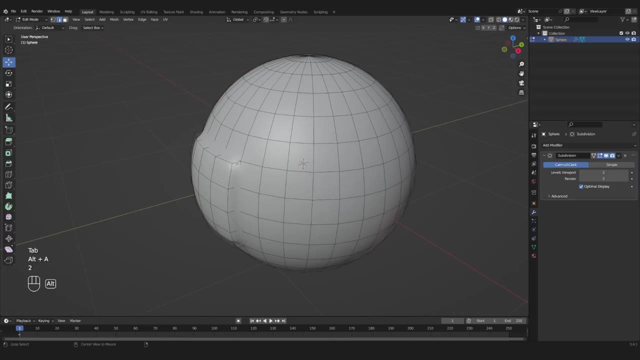 I'm using it very often, which makes the topology of my models look very clean. Tip number two. For this next tip, let's create a UV sphere and extrude some faces. If we add a subsurf modifier, everything gets smooth. so you might think to use creasing to sharpen the edges. 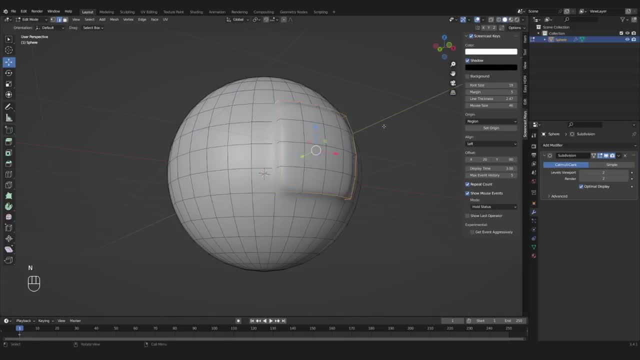 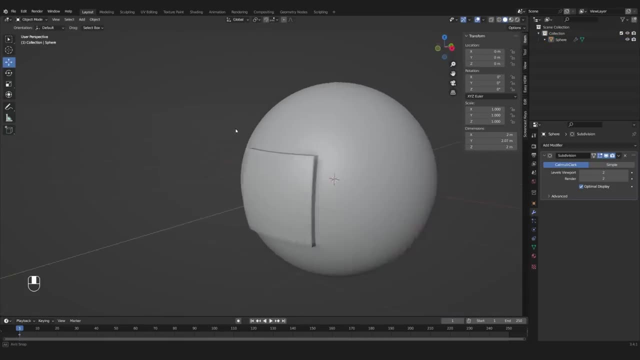 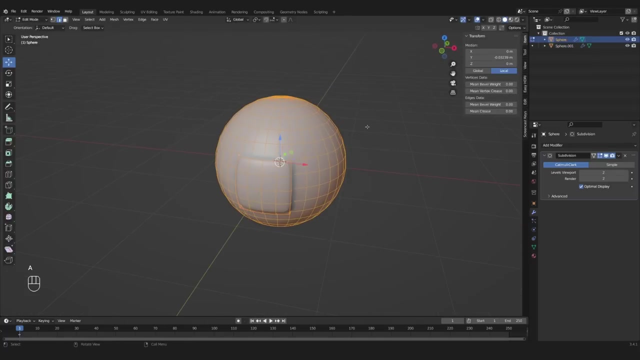 This might totally be enough for what you need it for In VFX, though this is not really the way to go. First of all, you can see that the smooth shading looks a bit weird on the edges. Also, creasing might cause problems when exporting the model to other software, since it might not be supported there or work a bit differently. 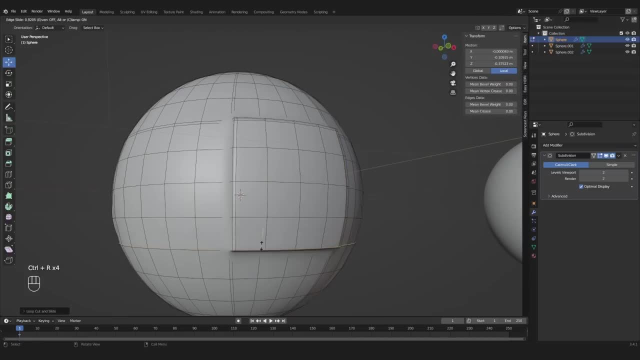 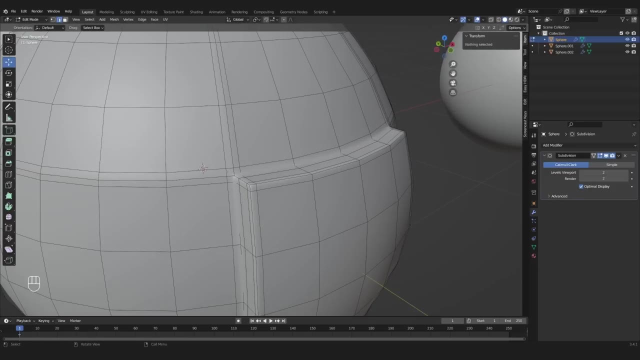 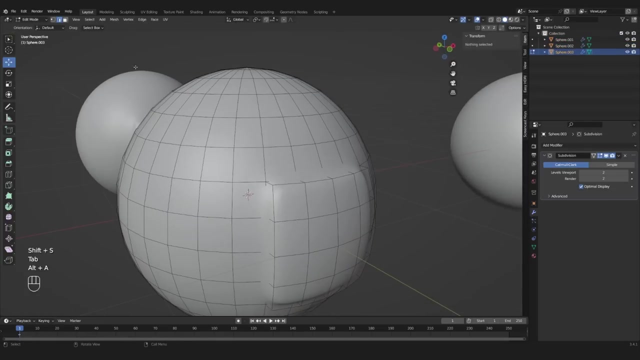 So let's instead use supporting edge loops. We now again have these corners which we know how to fix from the previous tip, But let me show you a different method for adding the support edge loops. Go to select- select sharp edges. Alternatively, you can select them by hand. 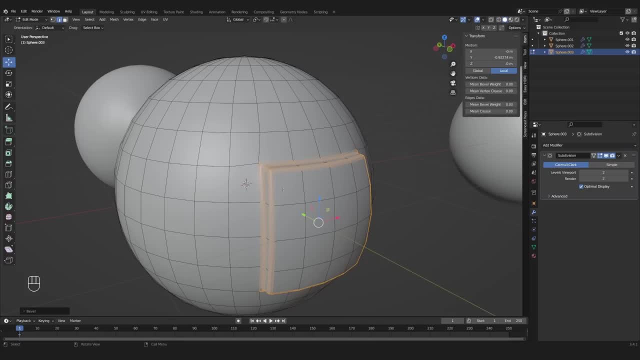 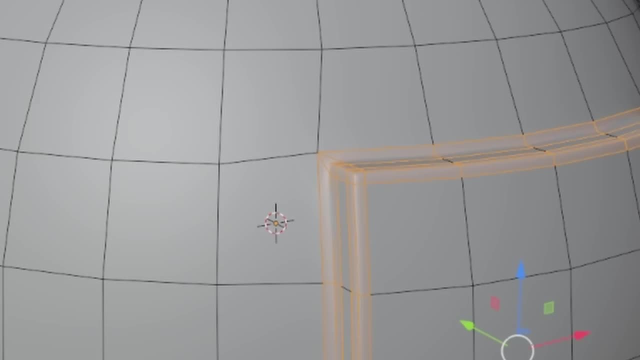 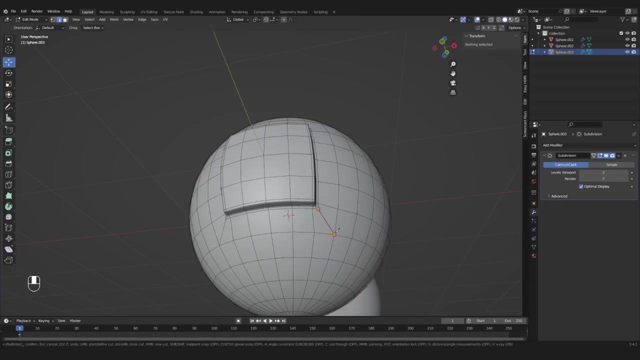 Now press ctrl B to bevel them In the settings. set the shape to 1 and the segments to 2.. Also, change the miter outer to arc, which will create this corner for you With the knife tool. you can now simply connect it like this, which will get you the same result as tip number one. 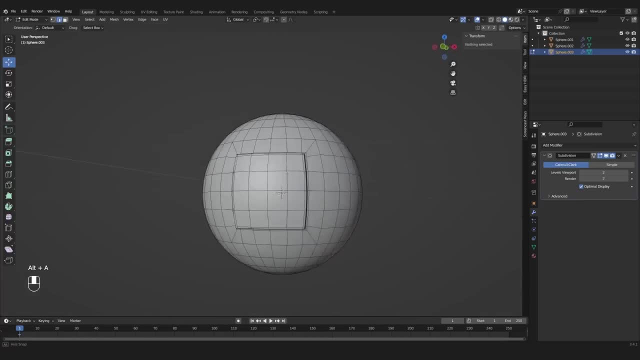 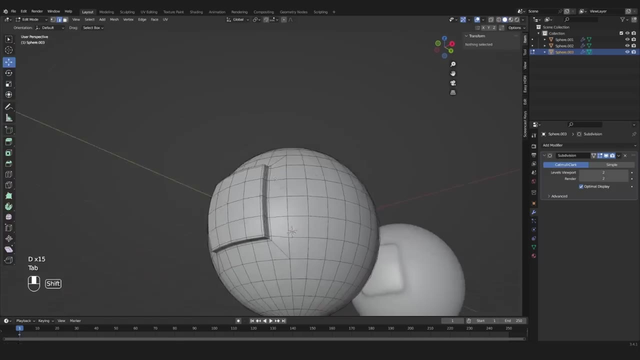 Now the topology looks fine, but you have this weird pinching in the corners. Obvious pinching is very common on curved surfaces. if you don't have enough topology, In most cases you can't eliminate it completely, but you can reduce it by increasing the tessellation. 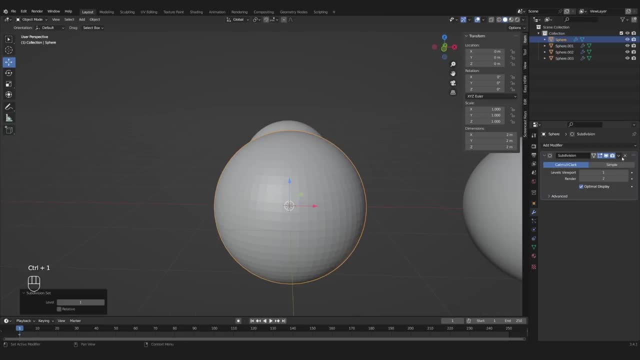 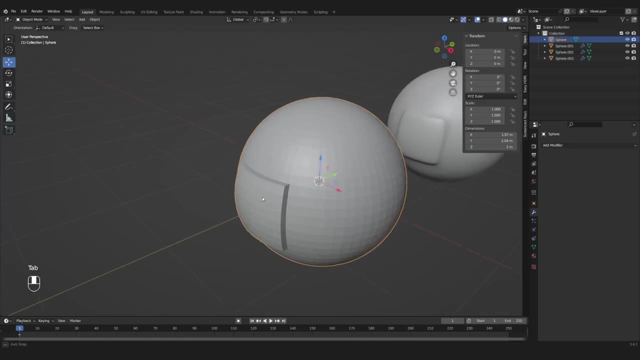 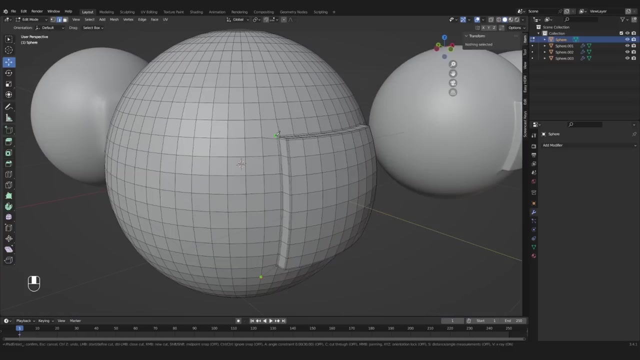 So let's add a new sphere, but this time apply one level of subsurf modifier first, Now as before, extrude some faces out, select sharp edges and bevel them. As you can see, there still is pinching, but it is much less obvious as before. 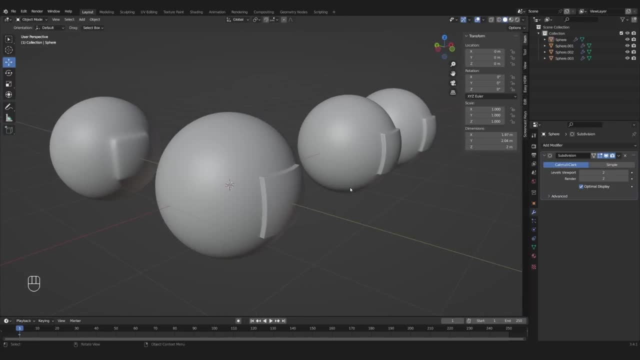 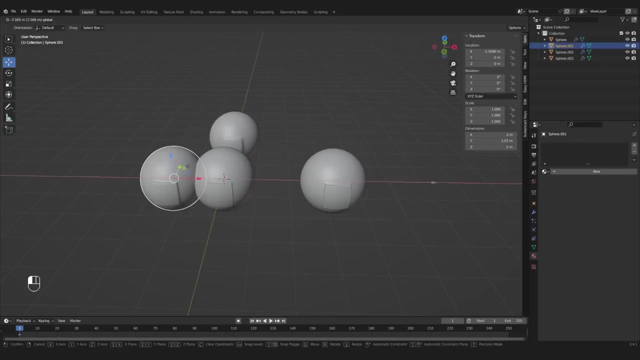 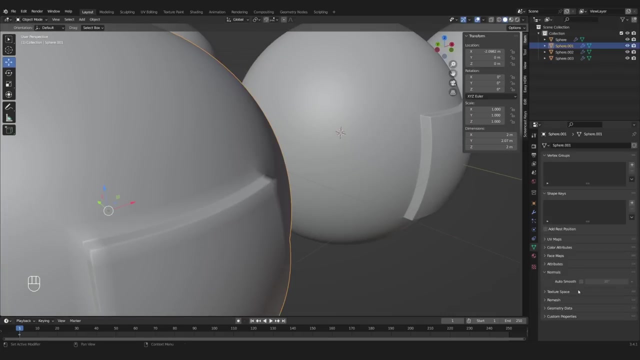 Of course, you could increase the topology even more, but depending on what material this object gets and from what distance it is seen, this might already be enough. If you now compare it with the creased version, it looks a lot cleaner. Of course you could enable auto-smooth, which will get rid of the weird shading. 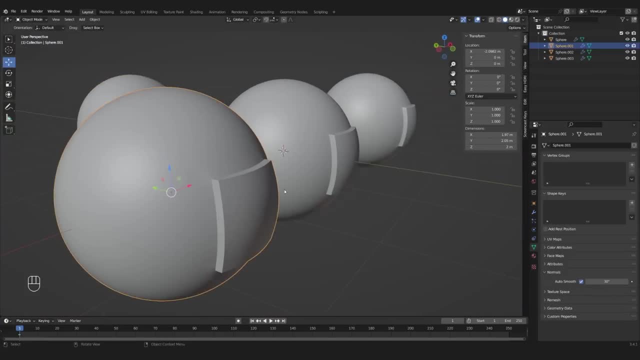 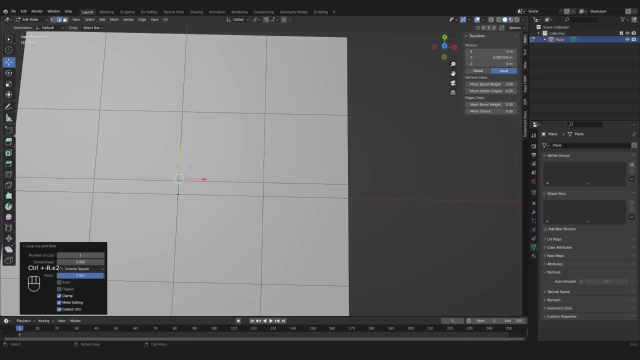 but this will also introduce some solidness. You can also add a little bit of pinching and make the edges perfectly sharp, which looks very unrealistic. Tip number three: Let's say you have this very even tessellated mesh, but for some reason you need a lot of topology in just one area. 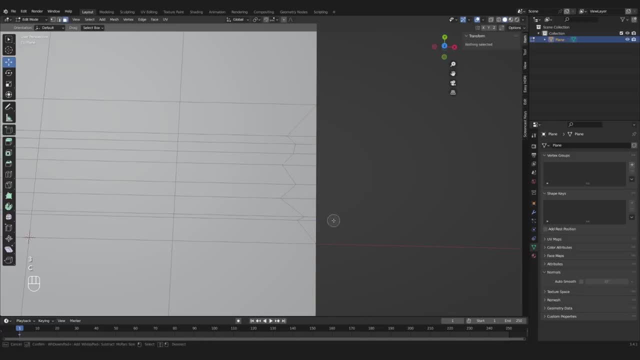 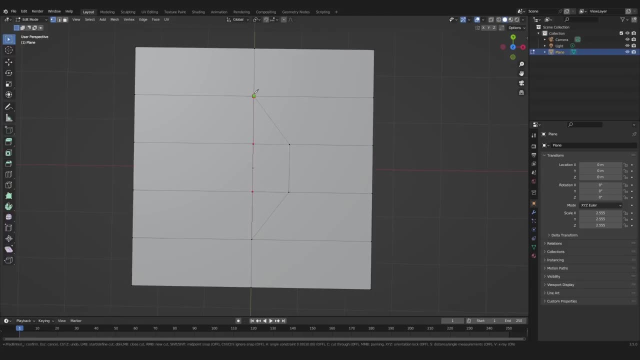 To have these extra edge loops not go through your whole mesh, there's a simple trick: Select the two neighboring vertices and move them back. Now connect the outer vertices together and remove the inner edges. Alternatively, you can use the knife and do it like this: 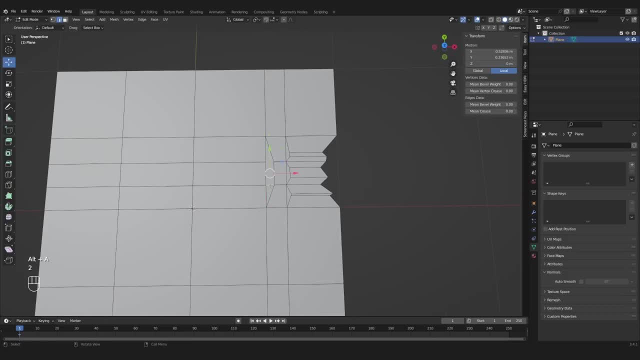 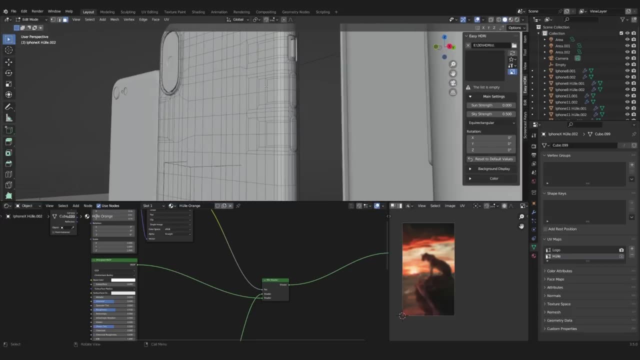 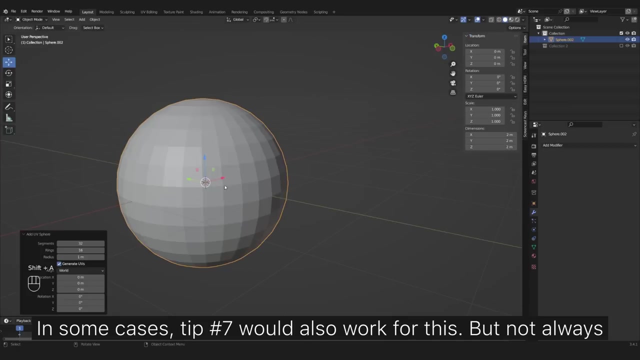 If that still isn't enough, you can just do it again. I used this tip in this example where I needed the topology for the buttons, but I didn't want it in the rest of the mesh. Tip number four. The next tip is not really an easy solution to a problem. 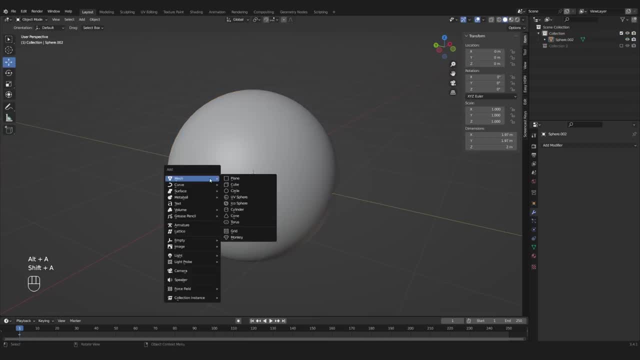 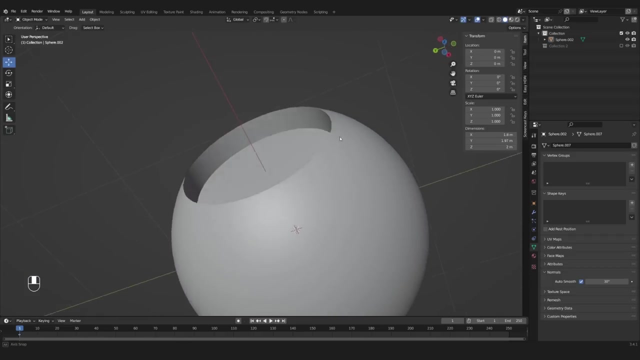 but requires a bit more work. So let's say you have a curved surface and you want to have a round cylindrical shape indented in there. So you might add a cylinder, set the vertices to a really high number and then just use the boolean modifier, set to difference, to eat away from the surface. 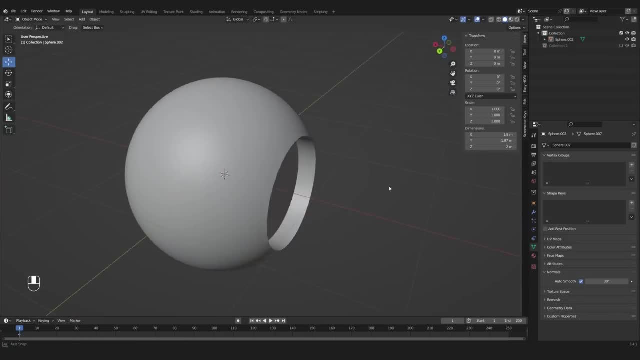 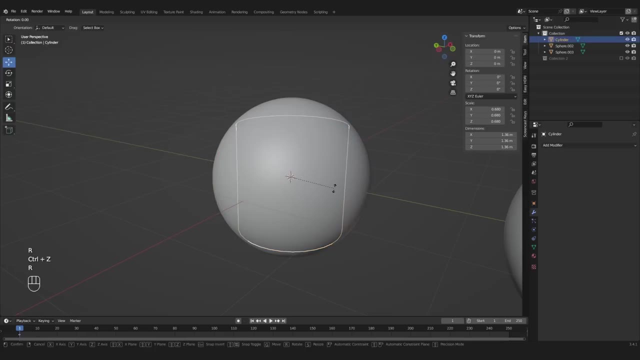 For a lot of cases, this is quite enough, but when using a subti workflow it isn't, So let's instead use a cylinder with much less vertices. I mostly try to stick with numbers that are a power of two If you move the cylinder in place. 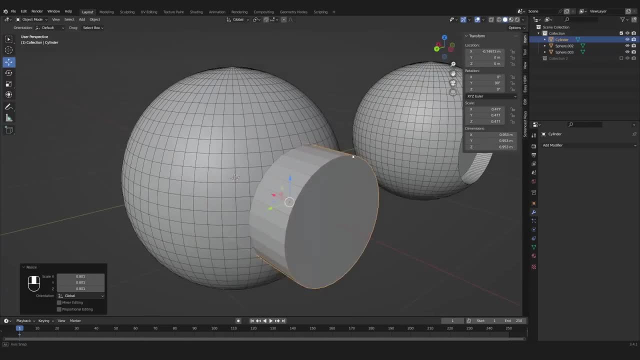 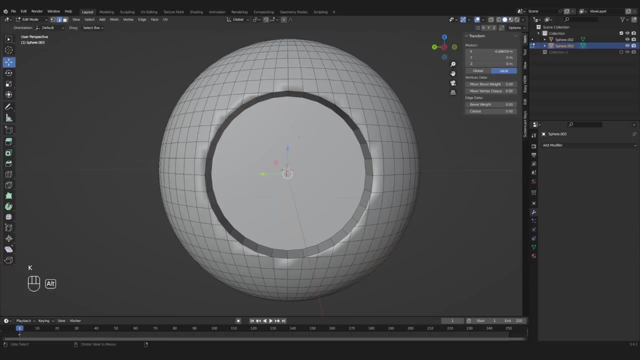 it should roughly have the same spacing between edges as the sphere. Now, again, use the boolean modifier set to difference. In this simple symmetrical example, I can use a mirror modifier to save some time. You might not be that lucky in your case. 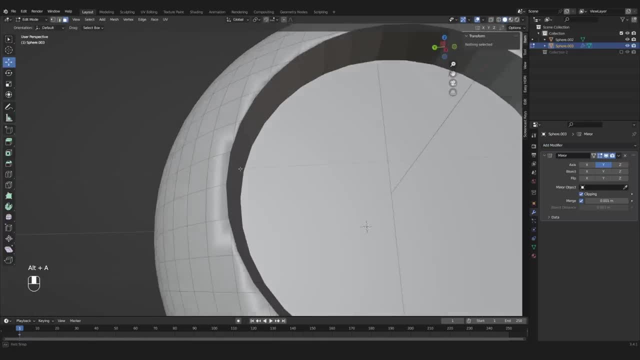 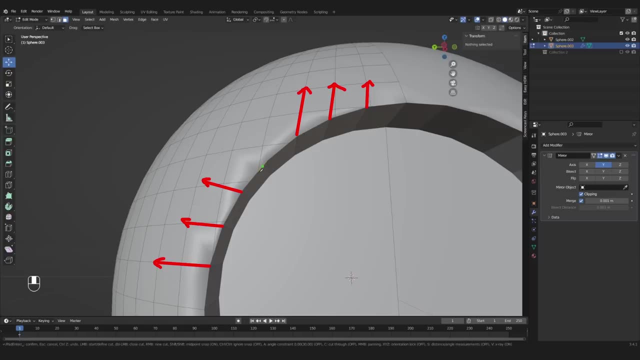 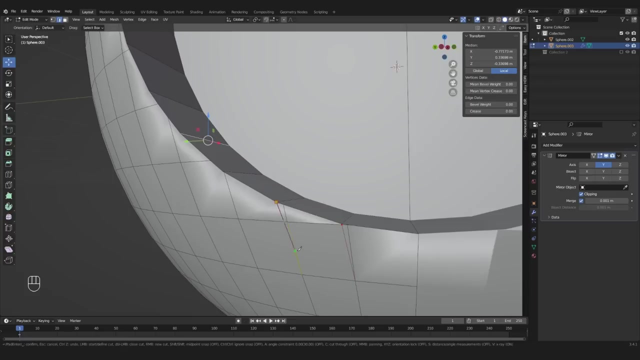 Let's now start by connecting the vertices of the cylinder to some close edge loops of the sphere On the left side. I want them to go left. on the top they should go up. Let's do the same for the bottom part. 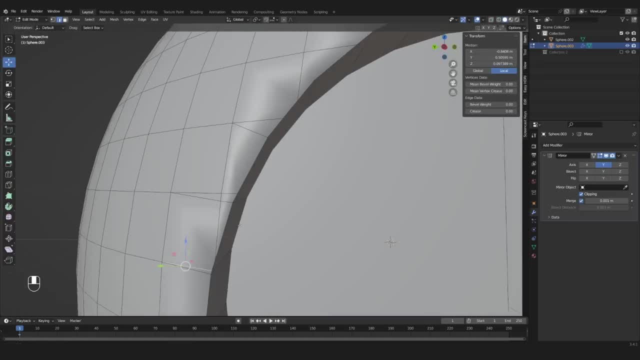 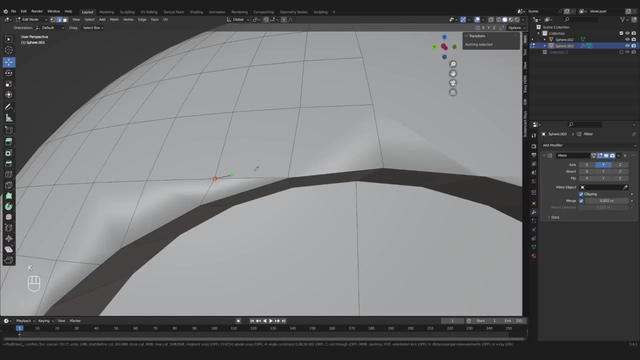 I can now delete some of the edges. I don't need anymore In this area. we could simply make a triangle out of this, but since it's very easy, I will just have it flow like this to keep it: quartz: Same below. 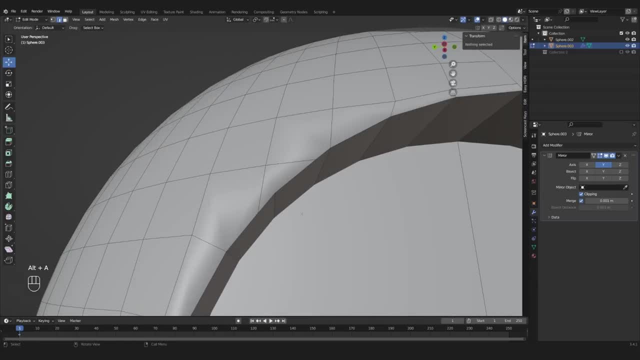 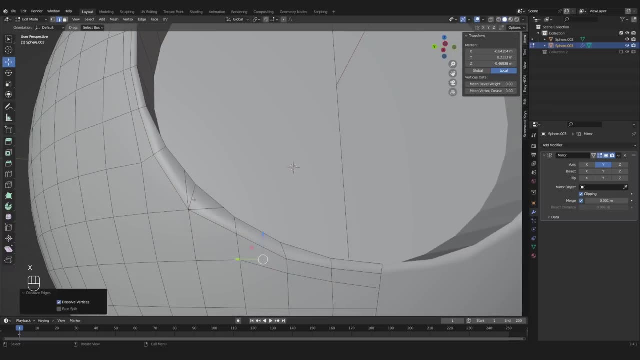 There is no step-by-step guide that always works in these cases, but after doing it a few times you start to see solutions to how your topology could flow. When you are done, you can bevel the edges with the shape set to 1.. 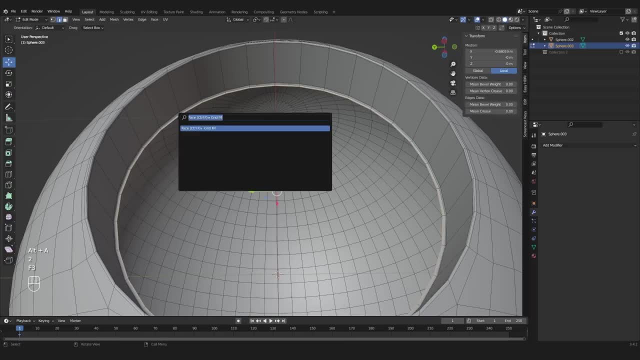 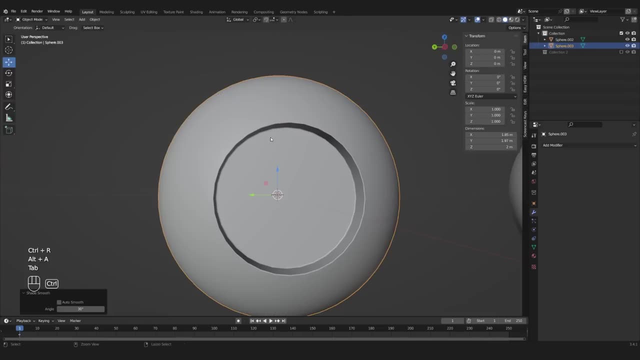 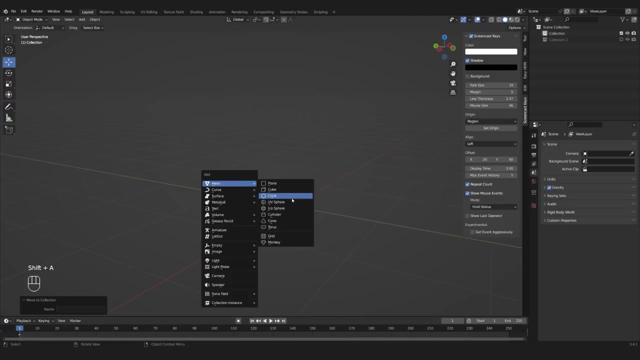 Let's apply the mirror modifier and use grid fill for the hole. We can now easily add a subsurf modifier and the mesh which stays in shape. Tip number 5.. The next tip, again, is a simple one. If you've ever tried to use a subsurf modifier on a UV sphere, 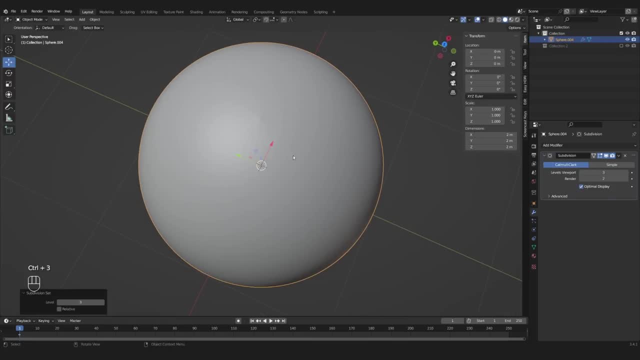 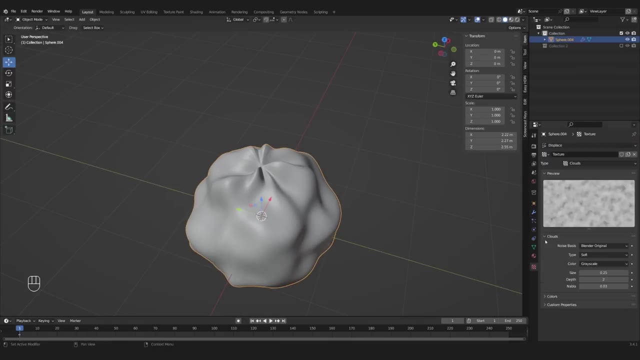 you might have noticed that the top and bottom will get this ugly star shape. If you add a displacement modifier with a simple cloud texture, this is even more obvious. There are two simple workarounds for that, Instead of using a UV sphere. 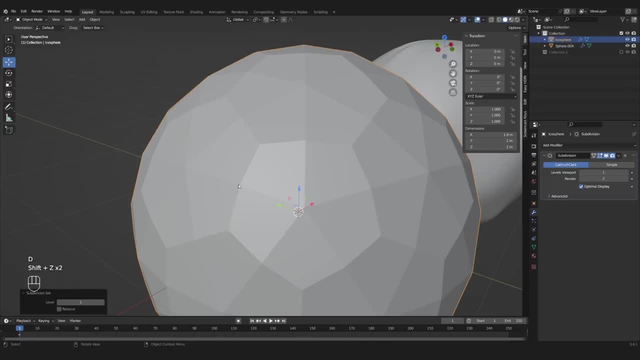 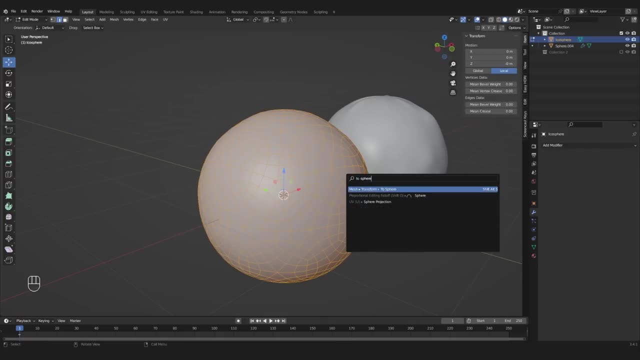 you could use an icosphere. When subdividing it, the stars turn into quads. We can apply the modifier and then use the two-sphere function to make it actually round. If you used the same displacement modifier, you can see that it works quite nice. 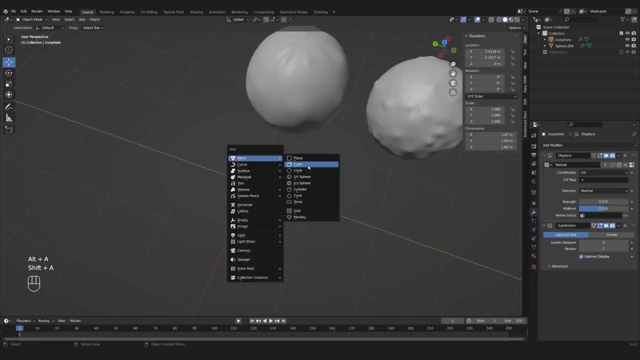 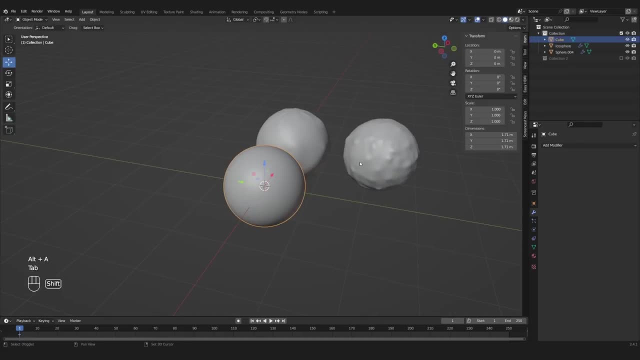 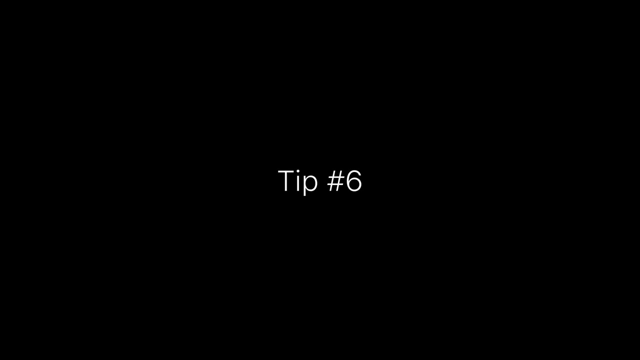 and we don't have this ugly star. Alternatively, you can subdivide a cube and again use the two-sphere function to make it perfectly round. This will get you an even tessellation without the weird problems on the ends. Tip number 6..